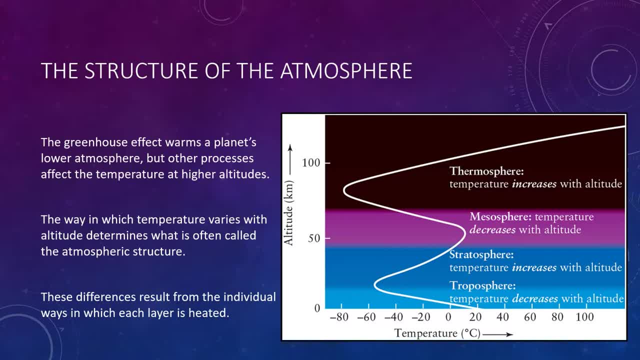 The key to understanding atmospheric structure lies in interactions between atmospheric gases and energy from the Sun. So this figure here, which you're going to see a variation of throughout many of the coming slides, shows you this temperature structure. So, from warmer temperatures on the right to cooler temperatures on the left, and altitude increasing as you move upward. 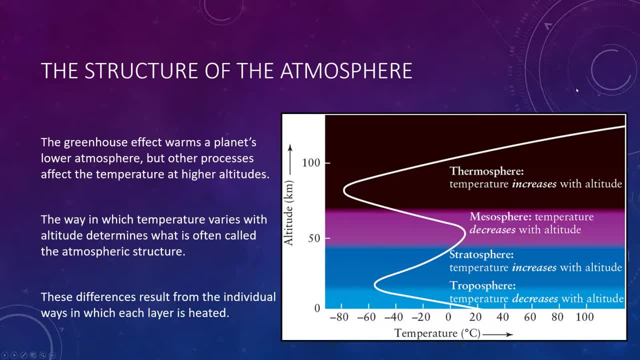 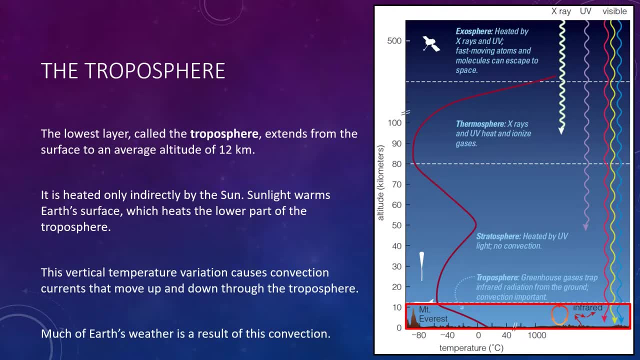 So we'll learn about each of these layers and why they have this structure that they do. So let's start from the surface, where we live, and we'll work our way upward. So the first layer, which you can see highlighted in red here, is the troposphere. 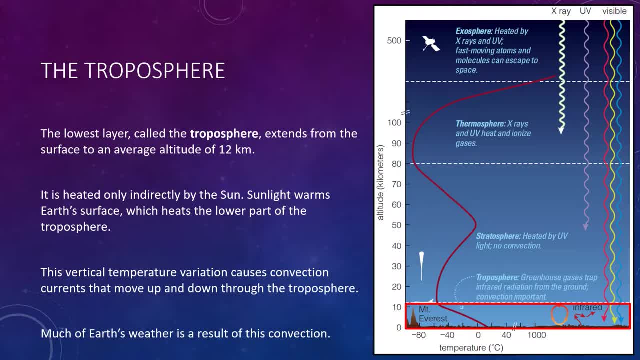 The lowest layer, which is called the troposphere, extends from the surface to an average altitude of about 12 kilometers, or roughly 7.5 miles. It is heated only indirectly by the Sun. Visible light passes through the atmosphere and warms Earth's surface, something we've discussed in our last video. 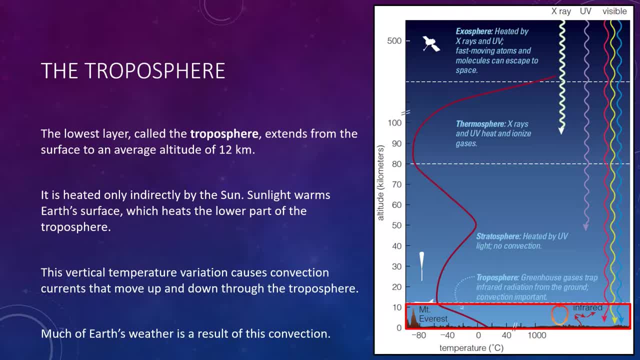 The ground returns the energy it absorbs by radiating in the infrared. Greenhouse gases absorb this infrared light and warm the troposphere. Because the infrared light comes from the surface, more is absorbed closer to the ground than at higher altitudes, which is why the temperature drops with altitude in the troposphere. 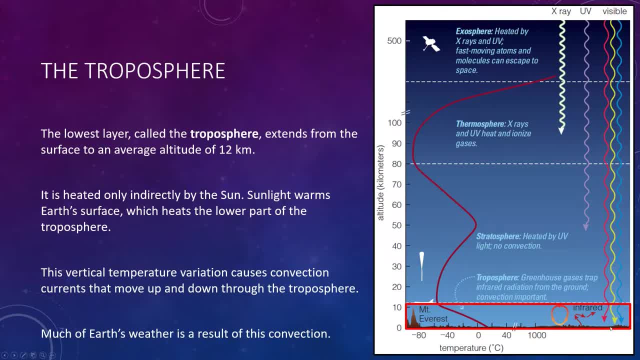 Alright. so we get visible light coming all the way down to the surface and then the surface emits that radiation via the infrared. But the greenhouse gases in our atmosphere trap that infrared radiation and heat the surface, So it's more efficient at the bottom. so our temperature declines as you move upward in the troposphere because of those greenhouse gases. 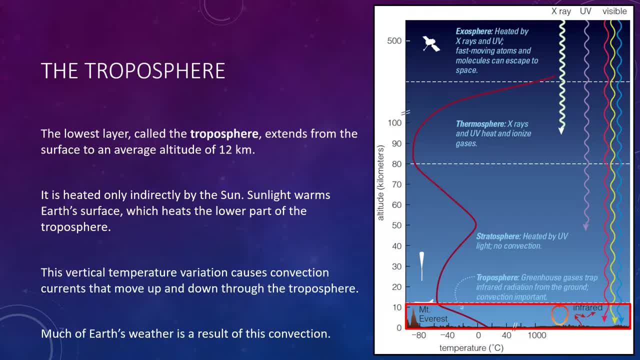 So, with that in mind, the drop in temperature with altitude, combined with the relatively high density of air in the troposphere, explains why the troposphere is the only layer in the atmosphere with storms. The primary cause of storms is the churning of air by convection, which you can see a little convection cell right here. 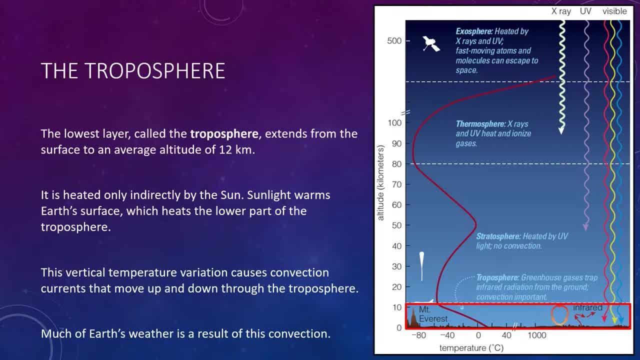 in which warm air rises and cool air falls. Recall that convection only can occur when there is a strong heating from below In the troposphere. that heating comes from the ground and drives convection. In fact, the troposphere gets its name from convection. 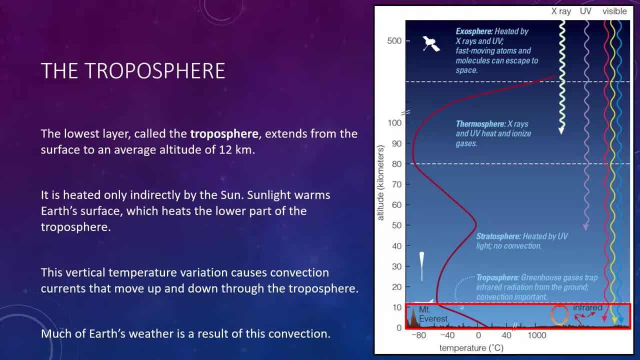 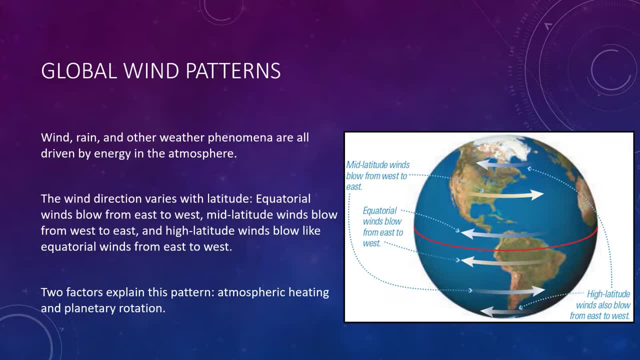 Tropos is Greek for turning. Wind, rain and other weather phenomena are all driven by energy in the atmosphere, which means only planets with atmospheres can have weather. Even then, weather varies dramatically among different worlds. Earth has the most diverse weather of the terrestrial planets, so we'll use it as an example of how weather works. 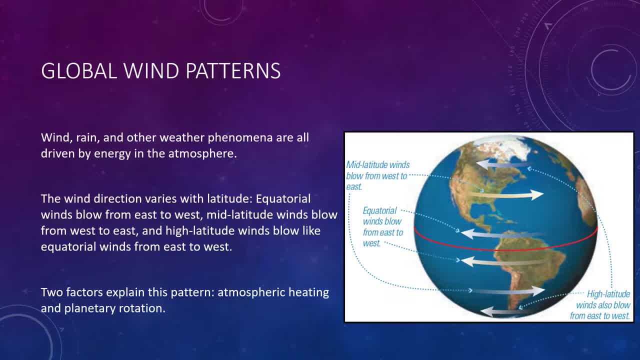 The wind's direction and strength can change rapidly in any particular place, but we do find distinct patterns on a more global scale. For example, winds generally cause storms moving from the Pacific to hit the west coast of the United States first, and then make their way eastward across the Rocky Mountains and the Great Plains before heading to the east coast. 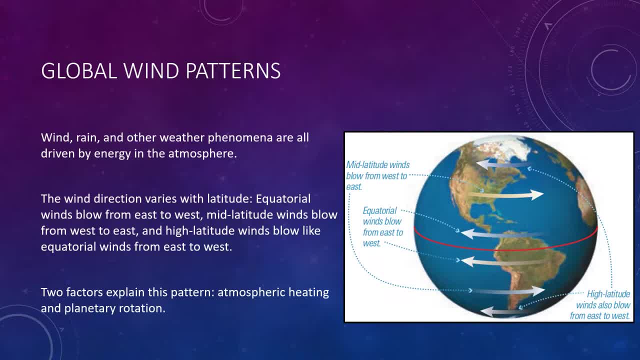 The figure here on the right shows Earth's major global wind patterns, or what we call global circulations. Notice that the wind direction varies with latitude. Equatorial winds blow from east to west, mid-latitudes blow from west to east and the high latitudes closer to the poles. 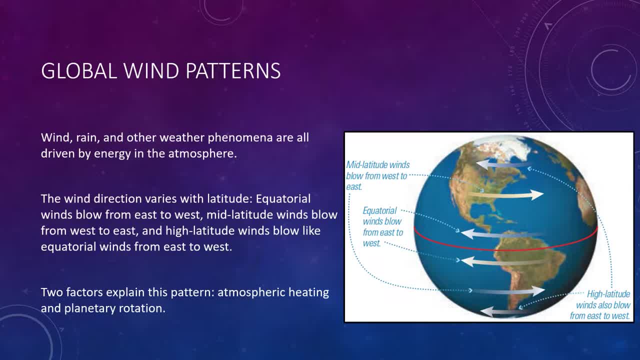 blow like the equatorial winds from east to west, and the high latitudes closer to the poles blow like the equatorial winds from east to west. Two factors explain this pattern: First, atmospheric heating and second, planetary rotation. So before we look at each of those in turn, let's just take a look at a quick animation or simulation of these global wind patterns. 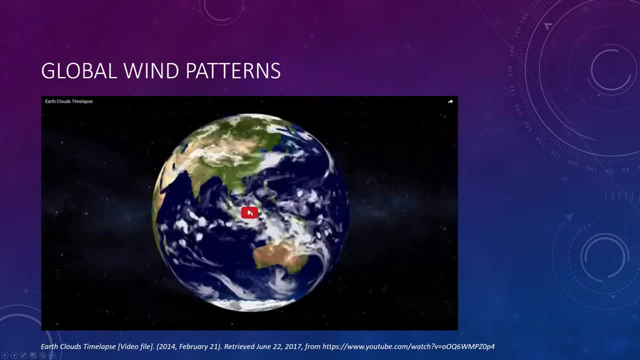 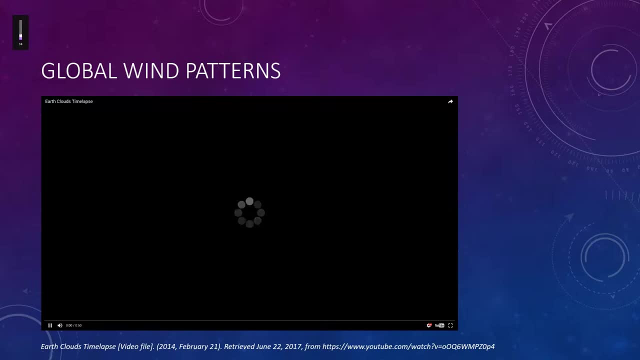 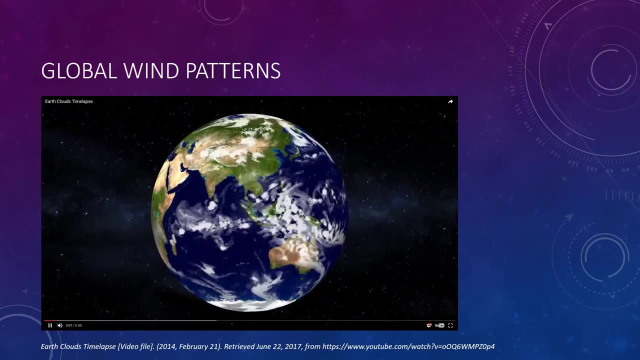 Excuse me, and now I have a reference here below, so let's just take a couple seconds to watch this so you can see these clouds in motion. If my Wi-Fi will connect here, There we go, So you can see the equatorial winds going from east to west. 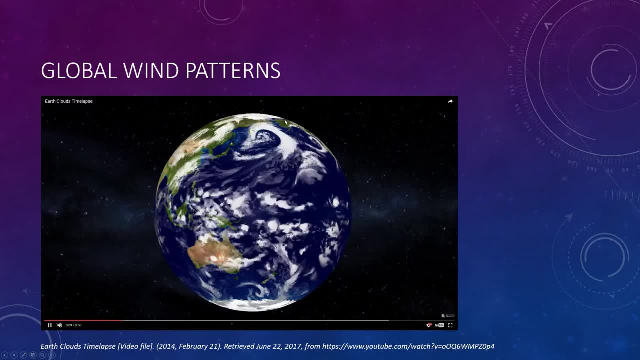 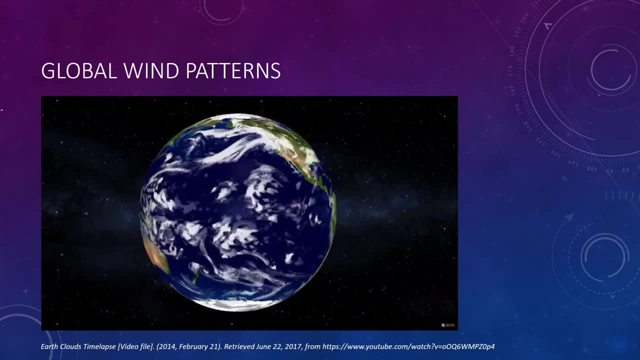 the mid-latitudes from west to east and the polar regions roughly going from east to west again. So we do see these patterns that persist throughout the entire continent, even though in some local area- perhaps you standing outside- the wind- could change direction at any point. 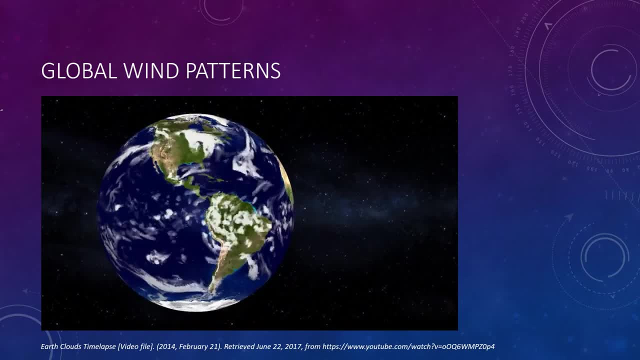 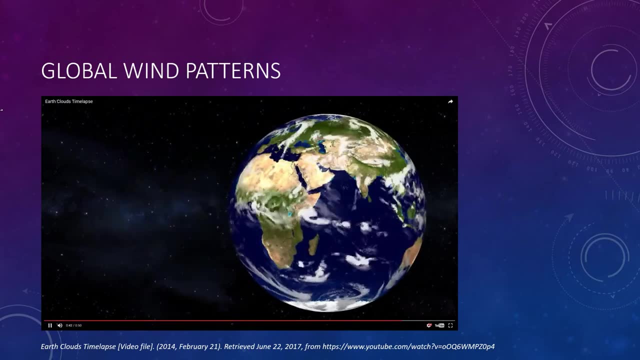 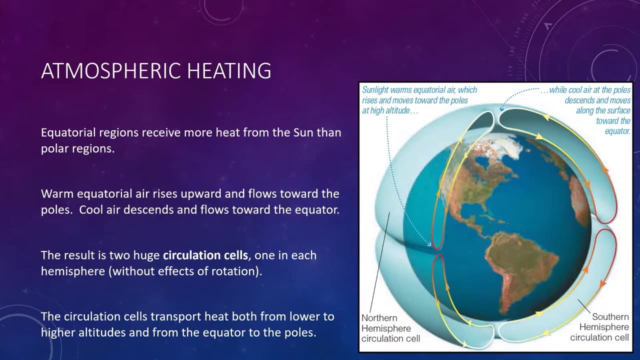 But in general we have these patterns. So let's take a look at those two causes for this in detail. Oh, I'm skipping along the video here. There we go. The first is atmospheric heating. Atmospheric heating affects global wind patterns because equatorial regions receive more heat from the sun than polar regions. 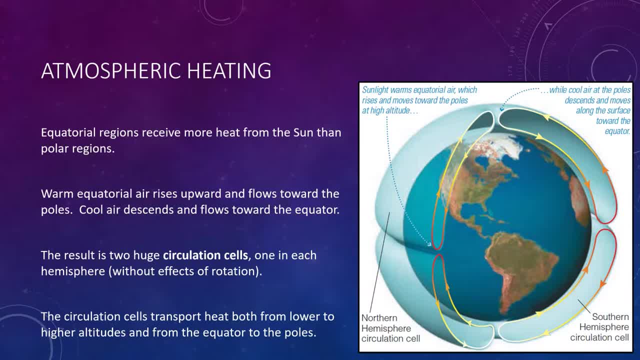 Warm equatorial air therefore rises upward and flows towards the poles, where cool air will descend and flow toward the equator. So the idea is it's warmer here in the equatorial, so the heat rises, but then it shifts toward the colder regions. 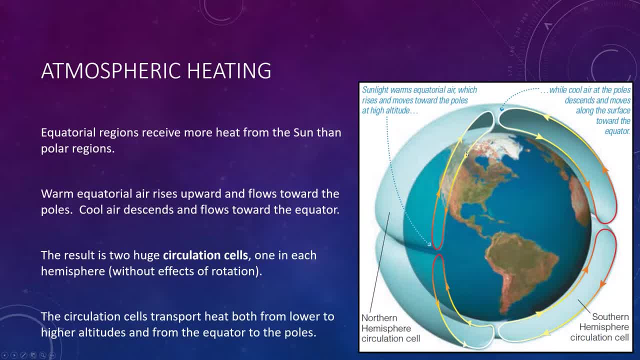 before it becomes more dense and sinks back down and you get these giant convection cells. So if Earth's rotation did not influence this process, the result would be two huge circulation cells, one in each hemisphere. So if we didn't have any rotation, 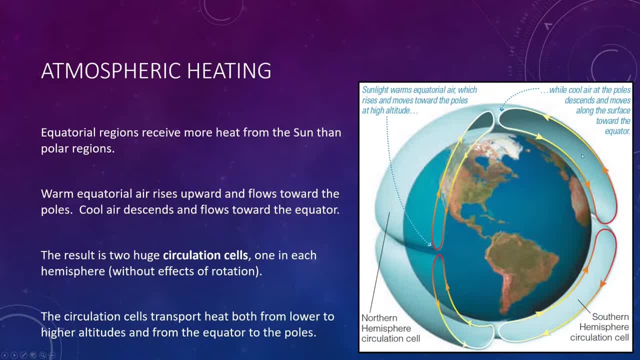 we would just have these giant patterns from north to south or vice versa. So if we didn't have any rotation, we would just have these giant patterns from north to south or vice versa. So if we didn't have any rotation, we would just have these giant patterns from north to south or vice versa. 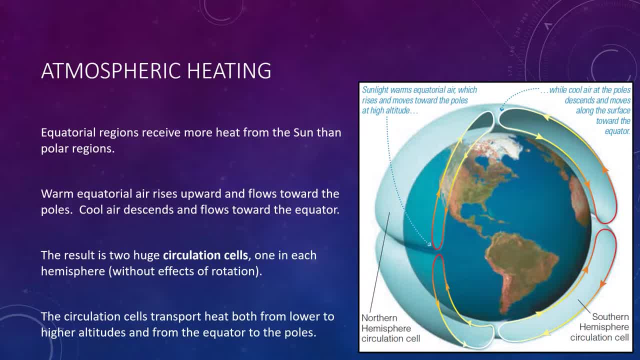 The circulation cells transport heat both from lower to higher altitudes and from equatorial to polar regions. They therefore make Earth's polar regions much warmer than they would be in the absence of any circulation. The same idea applies, to different extents, on Venus and Mars. 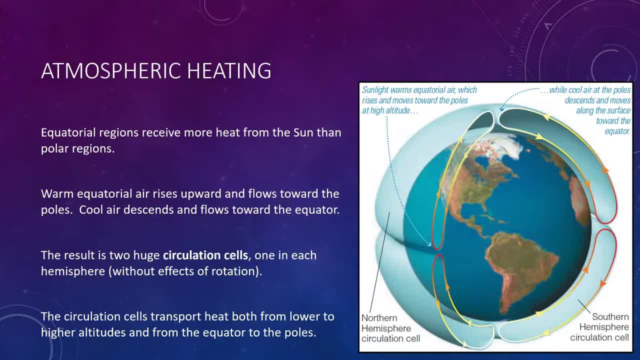 On Venus. the dense atmosphere allows the circulation cells to transport so much thermal energy that temperatures are nearly the same at the equator and the poles. On Mars, the temperature is nearly the same at the equator and the poles On Mars. the temperature is nearly the same at the equator and the poles. 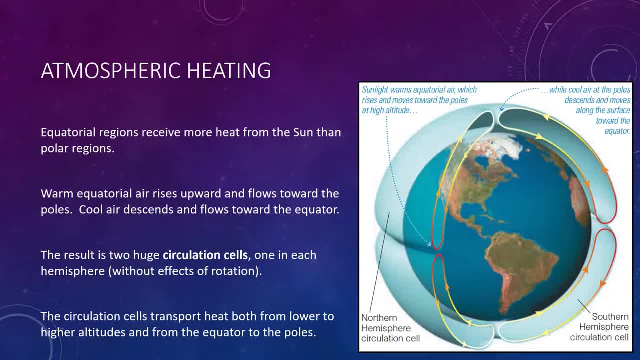 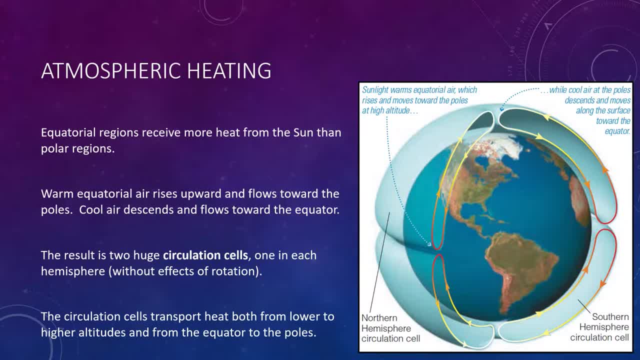 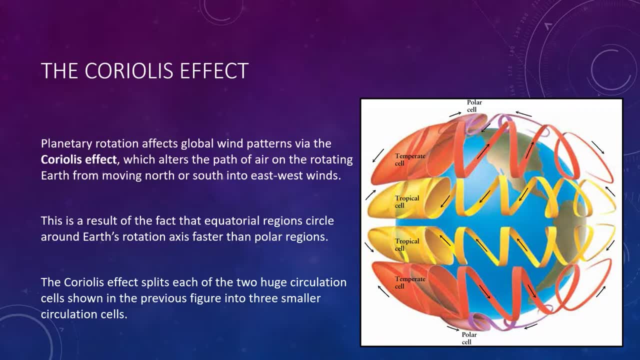 so just from heating we get this giant bipolar circulation cell setup. But there's one more thing that affects this Planetary rotation: affects global wind patterns through the Coriolis effect, which alters the path of air on the rotating Earth, which alters the path of air on the rotating Earth. 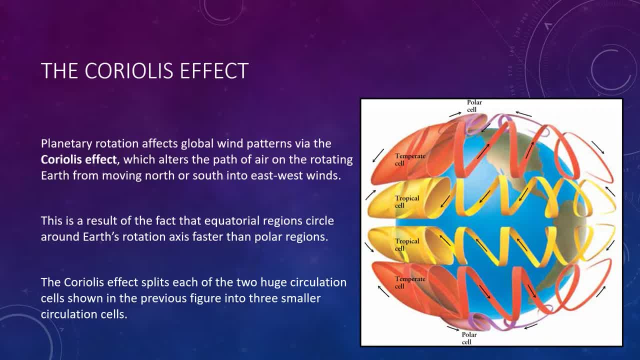 to east to west winds. Equatorial regions circle around Earth's rotation axis faster than polar regions because they have a greater distance to travel around the rotational axis. So basically we're saying winds have to move faster near the equator, Air moving away from 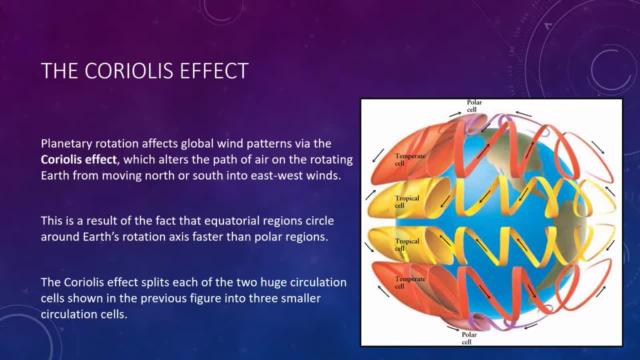 the equator therefore has extra speed that causes it to move ahead of Earth's rotation to the east, while air moving toward the equator lags behind Earth's rotation to the west. In either case, moving air turns to the right in the northern hemisphere and to the left. 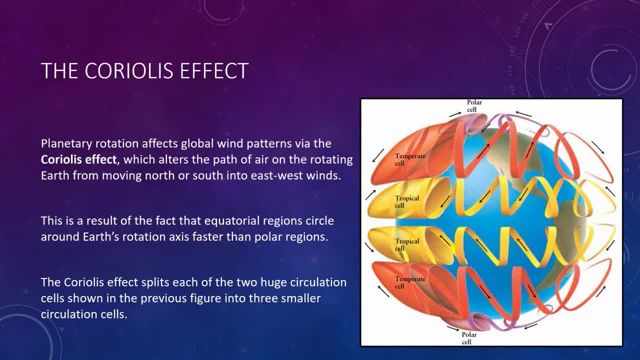 in the southern hemisphere, which explains why storms circulate in opposite directions in the two hemispheres. The Coriolis effect splits each of those two circulation cells that we saw in the previous figure into three smaller circulation cells that you can see in this image here on the right. 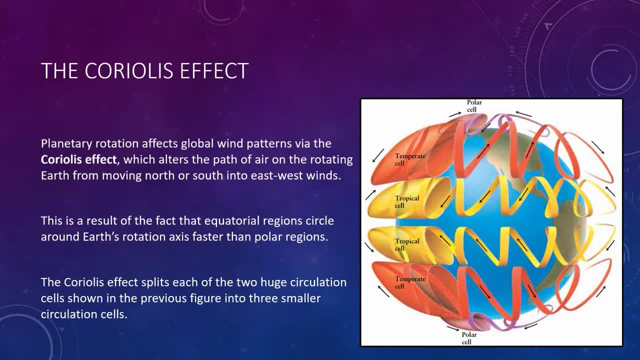 These motions explain the global wind directions. Notice that surface air moves toward the equator in the cells near the equator and near the poles. so the Coriolis effect diverts the air into westward winds. In contrast, surface air moves toward the poles in the mid-latitude. 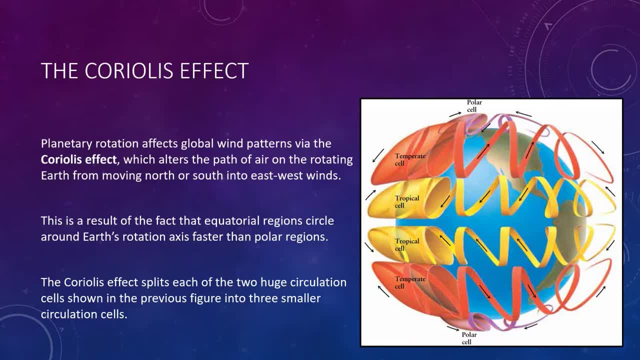 cells, so the Coriolis effect diverts its winds into blowing eastward. Stronger convection means more clouds and precipitation. That is why thunderstorms are common on summer afternoons, when the sunlight warmed surface drives strong convection. The linkage between clouds and convection. 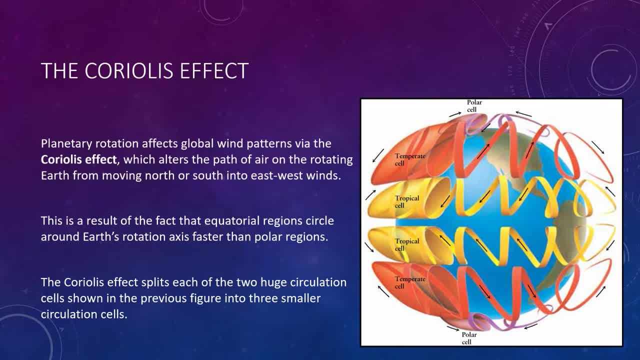 also explains why Earth has lush jungles near the equator and deserts at latitudes of 20-30 degrees north or south. Equatorial regions experience high rainfall because they receive more sunlight, which causes more of that convection. This high rainfall depletes the air of moisture. 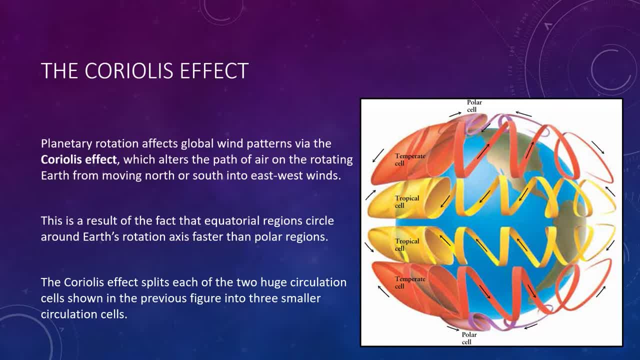 and Earth's circulatory cells carry it away from the equator, leaving little moisture to fall as rain in the latitudes of the equator. This is the result of the Coriolis effect 7. The Coriolis effect is the same as the Coriolis effect. The Coriolis effect is the 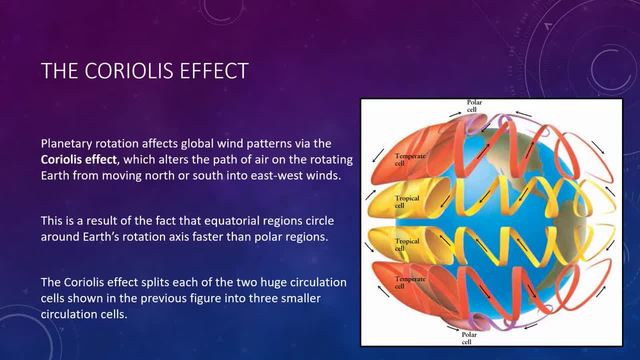 same as the Coriolis effect. The Coriolis effect is the same as the Coriolis effect, The Coriolis effect of the deserts. So kind of a unique way to look at this, how we can explain those forests and deserts. 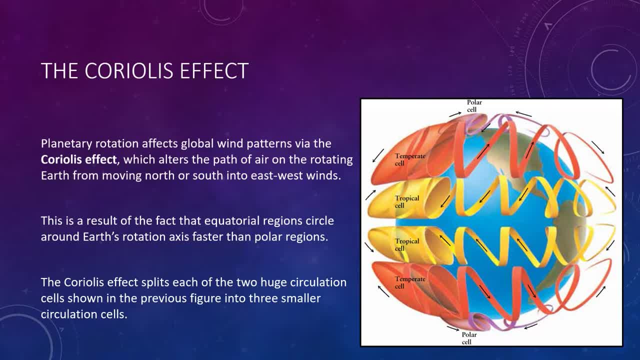 with a pretty simple concept, So you don't have to memorize the names of these different types of cells or anything, or exactly which way they move, but the general idea is important to grasp. All right, so that wraps up our discussion of the lower layer, the troposphere where we live in. 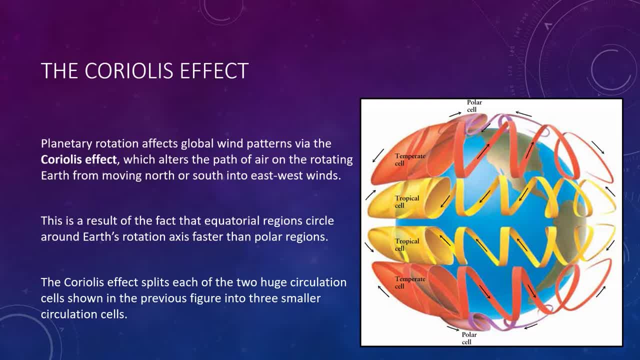 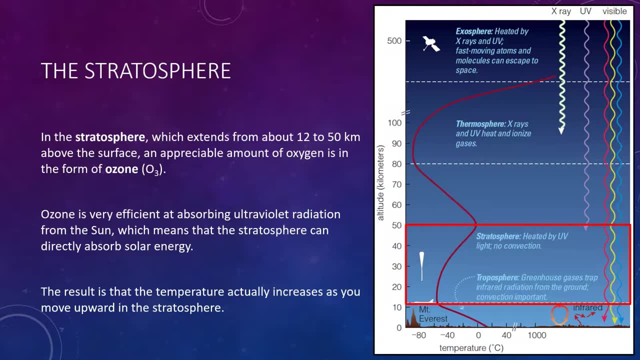 That was probably also the longest discussion on the layers, So let's move up one step to the stratosphere highlighted in red here on the right In the stratosphere, which extends from about 12 to 50 kilometers, or 7.5 to 31 miles above the surface. 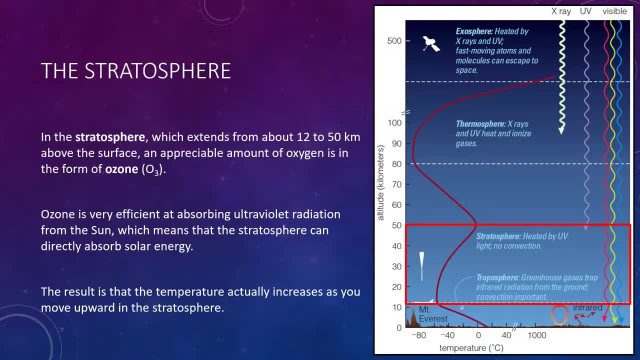 an appreciable amount of oxygen in the form of ozone, which is a molecule made of three oxygen atoms, exists. Ozone is very efficient at absorbing ultraviolet radiation from the sun, which means that the stratosphere can directly absorb solar energy. 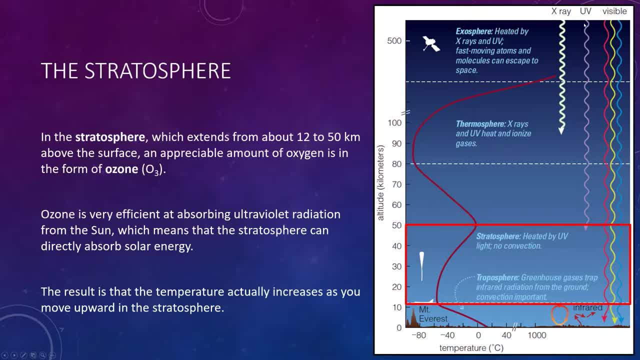 So that's what this is showing. in the image here, this little purple wavy line shows UV light coming in from the sun. Notice how it stops when it gets to the stratosphere. That's because it absorbs it- Most of this ultraviolet absorption and heating. 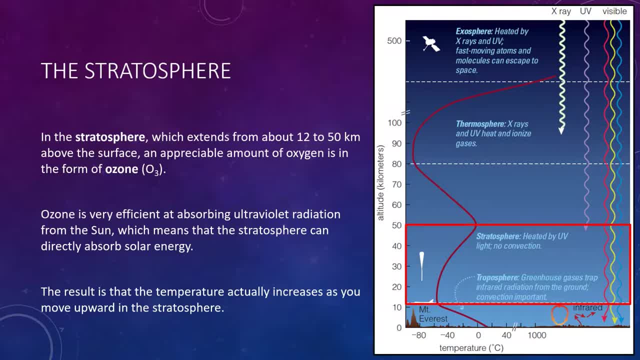 occurs at moderately high altitudes in the stratosphere, which is why the temperature tends to increase with altitude as we go upward from the base of the stratosphere Right. so we're absorbing energy at the upper parts of this region, so it's gonna be warmer there. 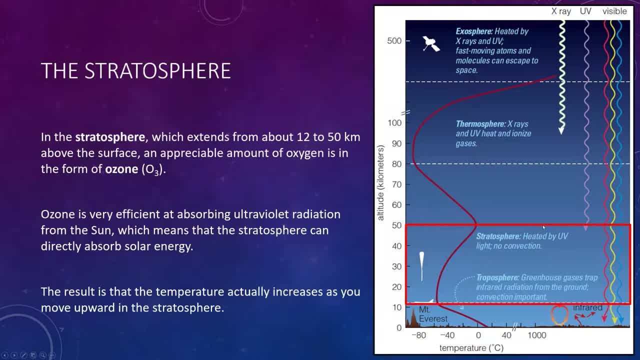 because of that absorbed energy. This temperature structure prevents convection in the lower stratosphere because heat cannot rise if the air above it is hotter. The lack of convection makes the air relatively stagnant and stratified, or layered, I'm sorry, stratified. 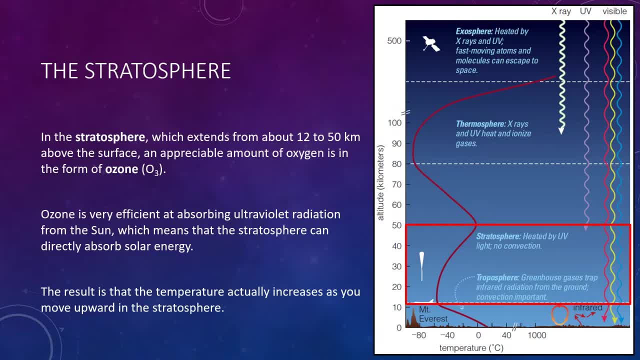 with layers of warm air overlapping cooler air. This stratification explains the name stratosphere. The lack of convection also means that the stratosphere has essentially no weather and no rain. Pollutants that reach the stratosphere, including the ozone-destroying chemicals. 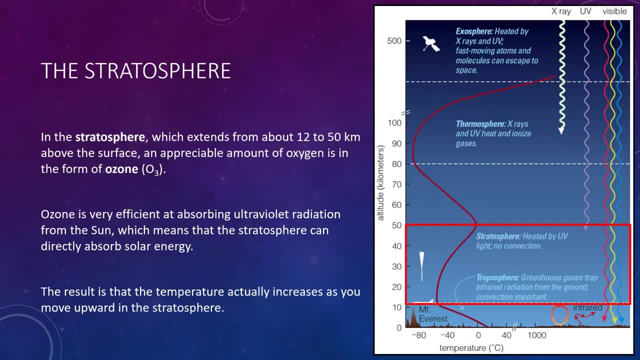 known as chlorofluorocarbons or CFCs, do remain there for decades. Luckily, we've been putting some regulations on that and we've seen a huge decline in CFCs. Note that a planet can have a stratosphere. 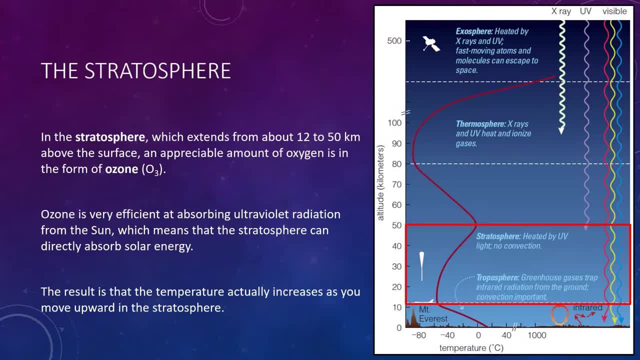 only if its atmosphere contains molecules that are particularly good at absorbing UV photons. Ozone plays this role on Earth, but the lack of oxygen in the atmospheres of other terrestrial worlds means that they also lack ozone. As a result, Earth is the only terrestrial world. 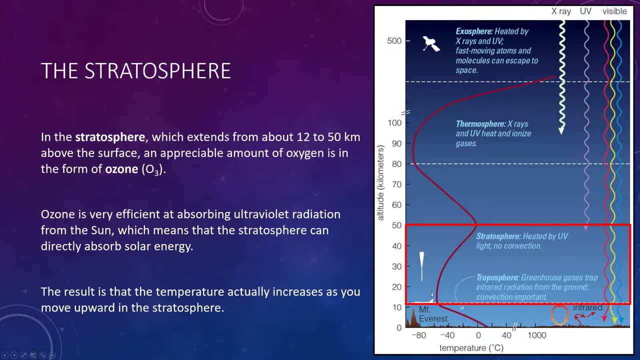 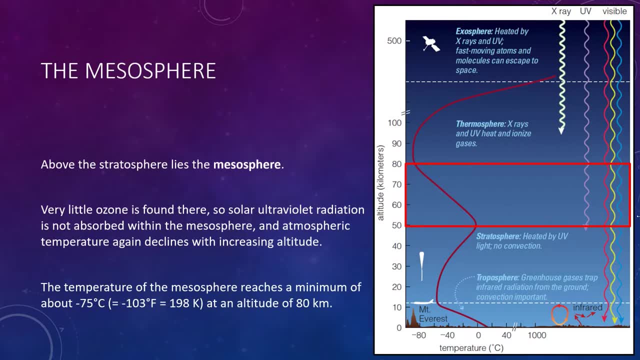 with a stratosphere, one of these layers where the temperature increases just above the troposphere. Next up is this middle layer here, which is the mesosphere. Above the stratosphere lies the mesosphere. Very little ozone is found there. 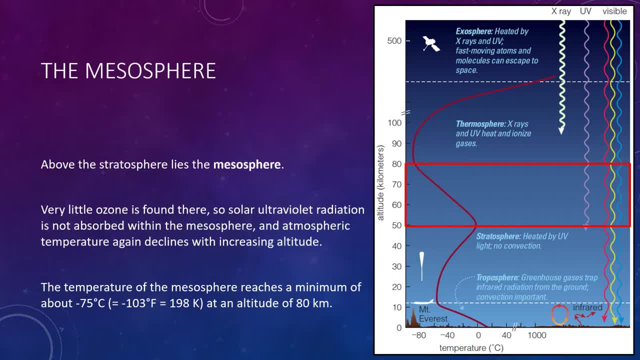 so solar UV radiation is not absorbed within this mesosphere and atmospheric temperature again begins to decline with altitude. The temperature of the mesosphere reaches a minimum of about negative 103 degrees Fahrenheit at an altitude of about 80 kilometers or 50 miles above the surface. 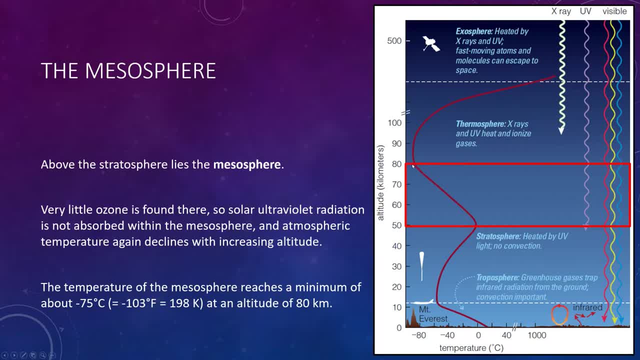 So we're talking very cold temperatures, about a negative 103 degrees Fahrenheit here, So nothing particularly interesting in the general sense happens here. UV invisible light passes right through it. Nothing is absorbed here, so the temperature just begins to fall back off. 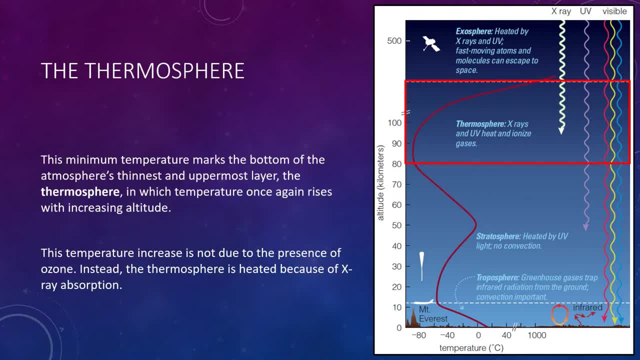 So, then, that brings us to the fourth layer, the thermosphere. This minimum temperature marks the bottom of the atmosphere's thinnest and uppermost layer, the thermosphere, in which temperature once again rises with an increasing altitude. The temperature increase. this time is due. 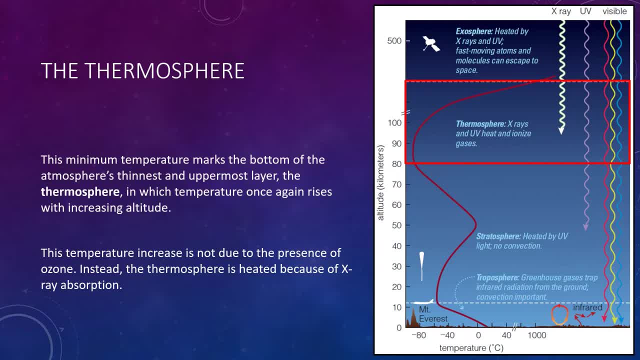